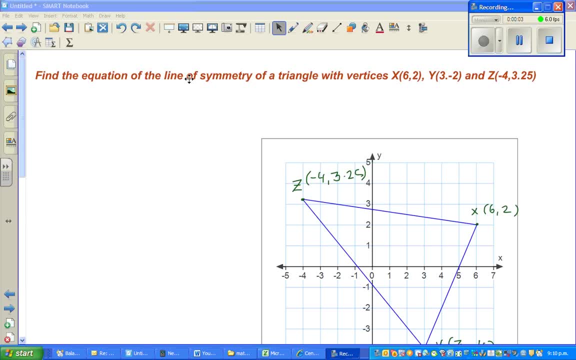 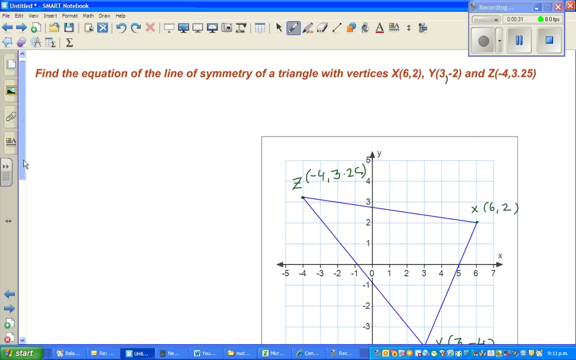 Let us look at this question, which is again an excellent question on the topic of coordinate geometry. So the question is like this: Find the equation of the line of symmetry of a triangle with vertices x, 6 comma, 2, y, 3 comma. this is comma 3 comma, negative 2 and y. sorry, 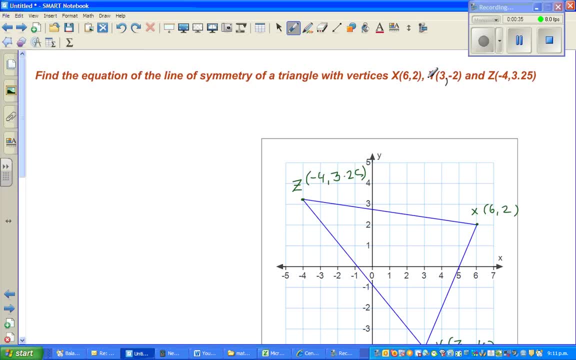 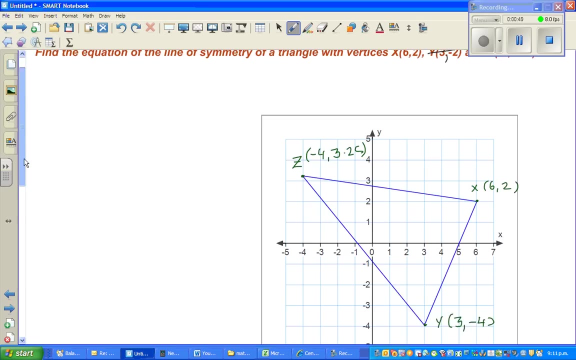 this should be negative 4.. Okay, so this is: y is 3 comma negative 4 and z is minus 4 comma 3.25.. I have plotted the point. So this is your x, which is 6 comma 2.. Okay, your y is 3 comma negative 4 and z is 3 comma. 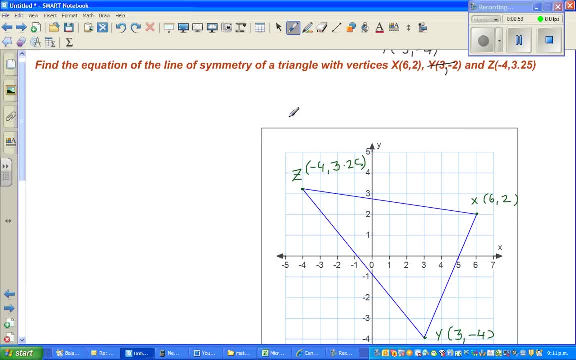 minus 4 comma 3.25.. Now to explain the line of symmetry, let me draw a triangle. Now. this is an equilateral triangle. Okay, suppose, yeah, okay, this is a triangle. Now to draw the line of symmetry. the line of symmetry is a line which cuts. 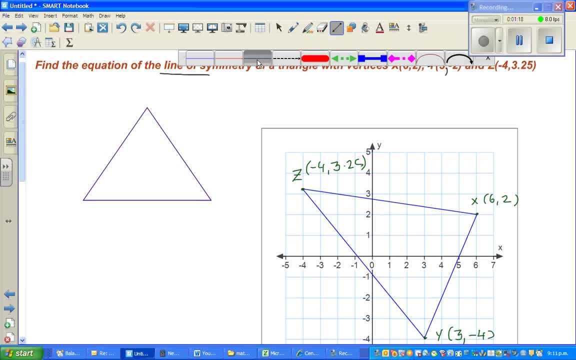 It cuts the triangle into two equal parts. So if I draw a perpendicular bisector like this, suppose a perpendicular bisector is a line which doesn't necessarily pass through the vertex, But here, in this case, it is passing through the vertex. So this is triangle ABC. 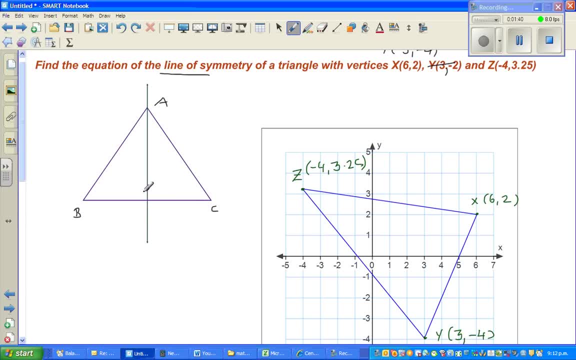 Okay, and this is a perpendicular bisector because this is passing through the midpoint. So this point, Okay, If you measure it. so these two are: suppose M is the midpoint And at M this line is forming a right angle. So this is a right angle. So you can understand symmetry. So 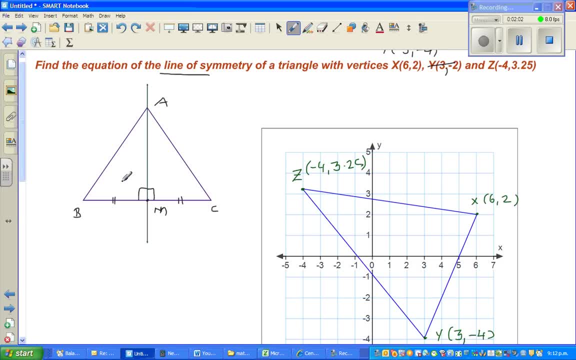 these two triangles. so if you flap this side onto this, so this will look like one same triangle. So in other words, these two triangles are identical. Okay, if you this is a, consider this as a mirror line. If you consider this as a mirror line, these two triangles. 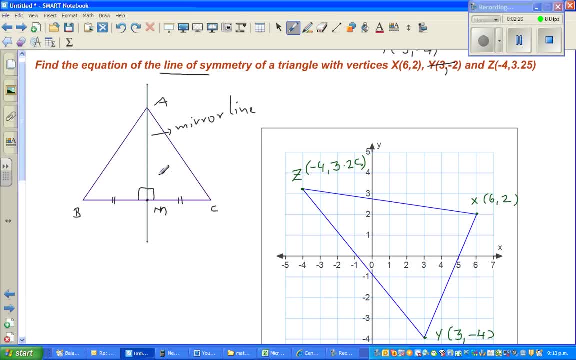 are equal. Okay, So this is a line of so. so line of symmetry of a triangle should be a line which is passing through a vertex and it also perpendicular bisector. So then you can say: this triangle, this line which is perpendicular to the left. 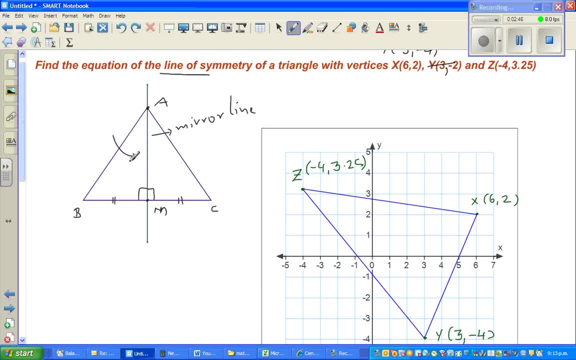 There one is parallel That one, And then you have oneucks and one forgotten. So the bisector, now it's called perpendicular bisector, the word itself. there are two words. one is it should be perpendicular and it should bisect the side opposite to a. suppose this is the side opposite to a, so this line is perpendicular. 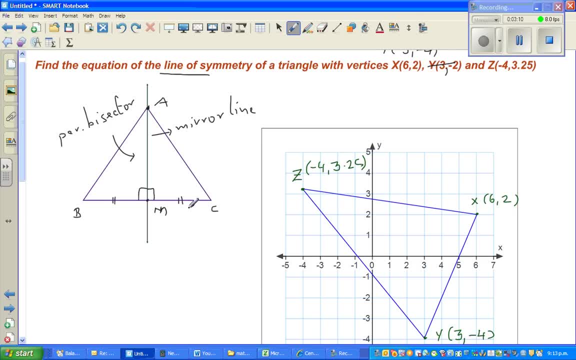 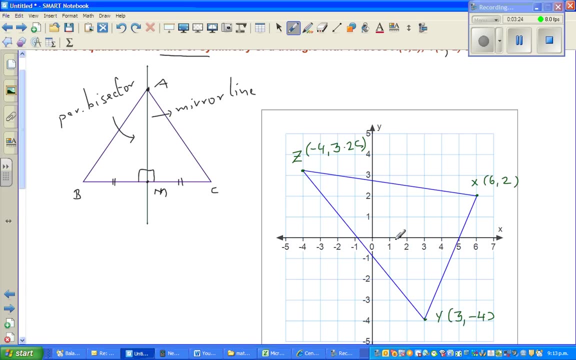 bisect is passing through a and is bisecting b. so if these three, if it has these three characteristics, then you can say this is the line of symmetry of the triangle and this triangle. this is not as neat as this triangle, so you would find make a guess of a line which would exactly pass through one of the. 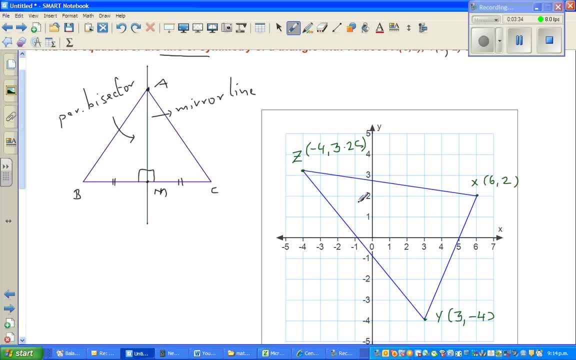 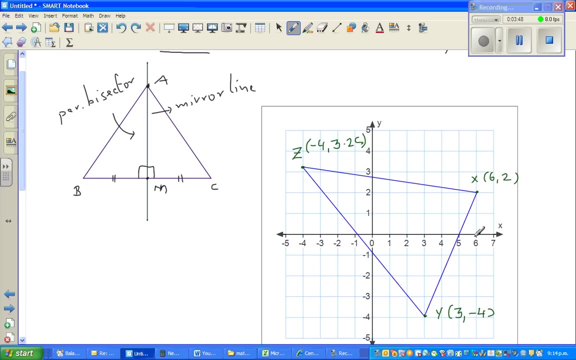 vertex and pass through the midpoint and also becomes a perpendicular bisector. so let us make, say, guesses here. so let's first: perpendicular bisector has two possible: the midpoint, so first an easy midpoint. so to find the midpoint of XY, you add the X intercepts, sorry, X coordinates. so 6 plus 6 plus 3 is 9, and 9 divided by 2 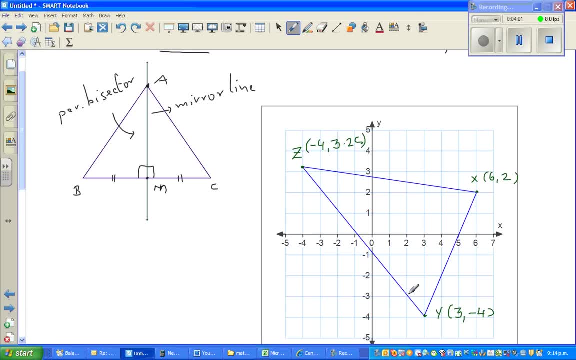 is 4.5. so your 4.5, sorry. 6 divided by 6 plus 3 is 9, yeah, and divided by 2 is 4.5. so 4.5 comes somewhere here. okay, now to find the Y coordinate: is 2 plus. 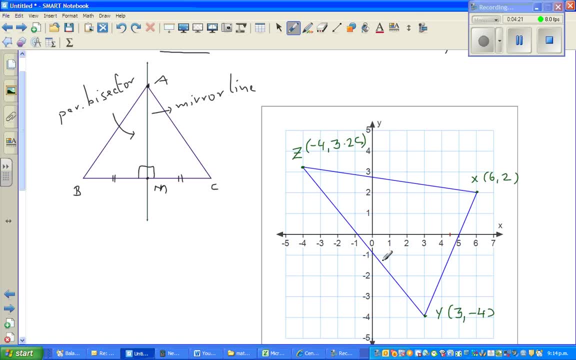 negative. 4 is negative 2 divided by 2 is negative 1, so this is your negative 1, so the midpoint is this point. okay, so this is the- let us call that M, which is a midpoint, and the coordinate is 4.5 comma- negative 1. 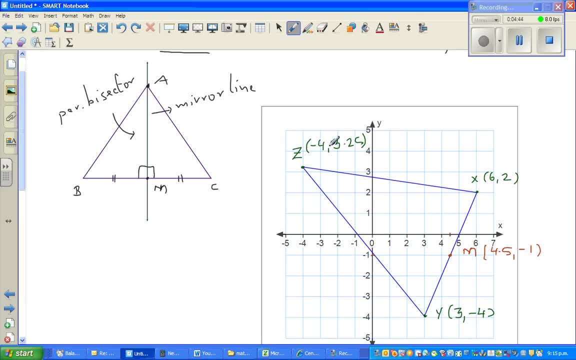 so what's the midpoint of this? you add the X intercepts, so X coordinate. I keep saying X intercept, so negative. 4 plus 6 is 2, 2 divided by 2 is 1. so this is the midpoint. okay, this is a midpoint. so this is 1 comma 3.5. so let me use a. 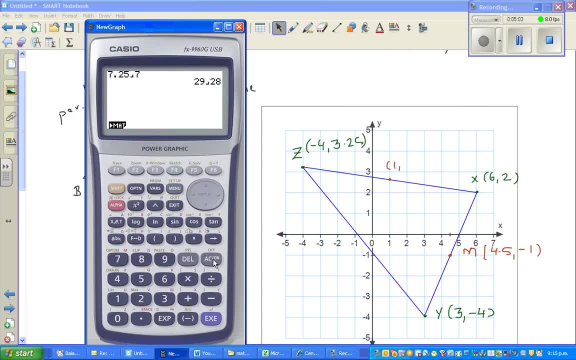 calculator. I'm a bit tired now. so 3.25 plus 2, that is 5.25. divided by 2, 2 is 2.625, 5, right? so this look looks like 2.6 to 5. yeah, that's fine. so this: 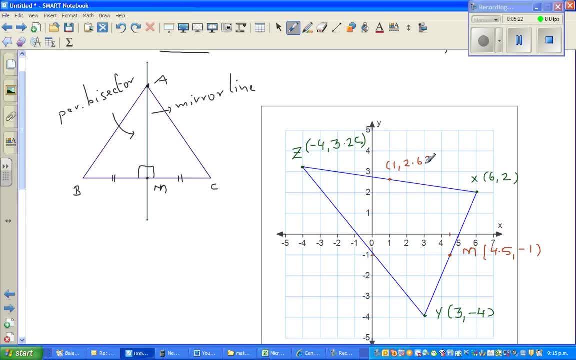 is 1 comma, 2.6, 25, and the midpoint of this will be somewhere here I'm making a guess. so minus 4 plus 3 is minus 4 plus 3 is negative. 1 divided by 2 is 0.5. 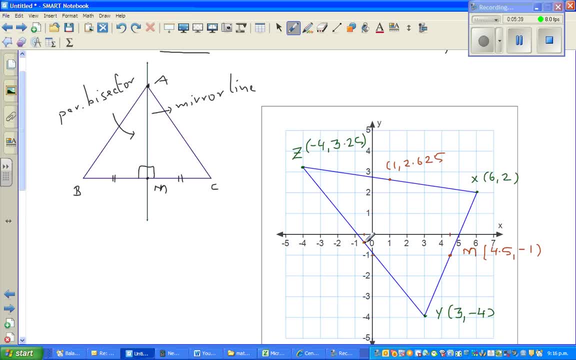 so this is 0.5. so midpoint comes somewhere here. so this is, say, my N and so this is my O, and the coordinate would be: this is 0 minus 0.5 or minus half. let me write minus 0.5. yeah, this coordinate will be 0.5 comma. 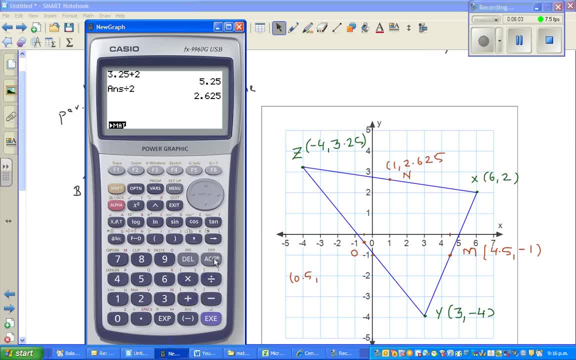 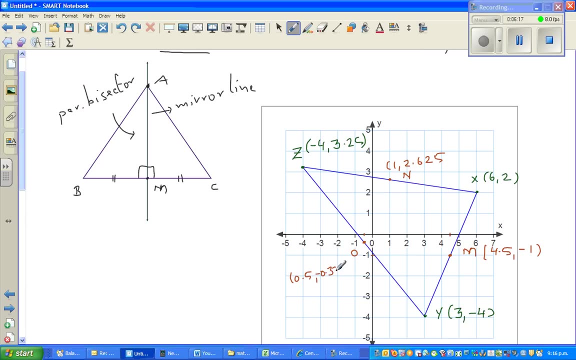 to find the Y coordinate. I'll use the calculator. so that is 3.25 plus negative 4, which is, and then you divide by 2, which is negative 0.375. so negative 0.375 now if you draw a perpendicular. so, as I said, the the, the line of symmetry of the 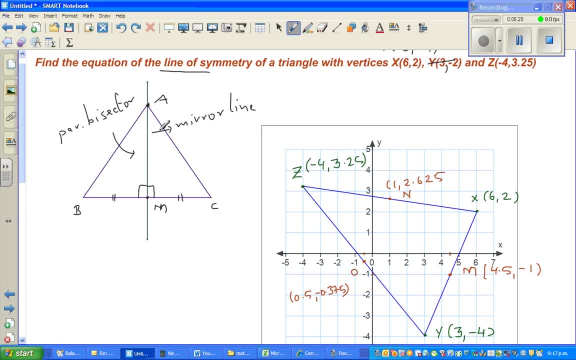 triangle should be a line which is passing through a vertex and is also the perpendicular bisector of the opposite side. so I'm making a guess: if I do this, I will get a line which is passing through a vertex and is also the perpendicular bisector of the opposite side. so I'm making a guess if I do. 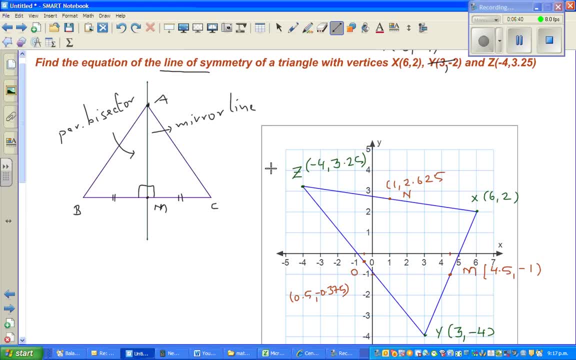 draw a perpendicular from Z to XY, it will pass through the midpoint. I'm making a guess. I have to prove it first. what I'm going to do is I'll have to find it's a good guess. so it's all you could do: all the three side, find the. 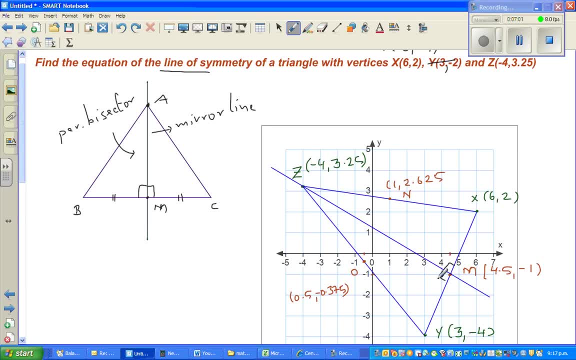 perpendicular bisector of all the three sides. and here I'm making a guess, a good guesses. this seems to be perpendicular. it's passing through the midpoint, is also passing through the vertex. first we'll have to find the equation of this line, okay, and then show that on this line this point does lie. okay, now to 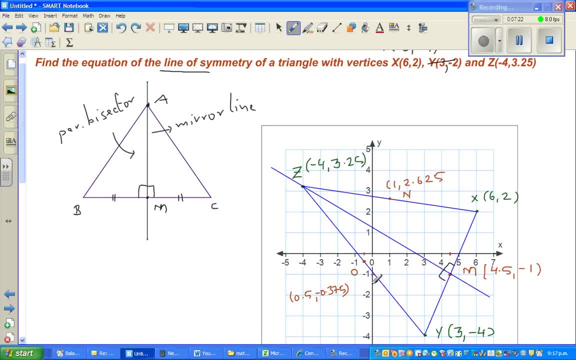 find the equation of this line, you have to first find the equation of XY. so let me find equation of XY, for which we'll have to find the gradient of XY. so I'll write like this: MXY is rise over run, so rise is from minus 4 to 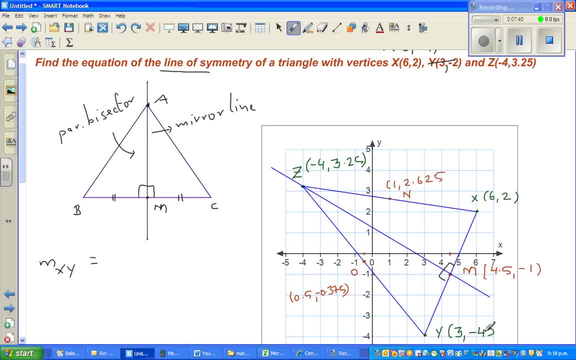 I'm going from Y to X, so it's minus 4 to 2. minus 4 to 2, there's a rise of 6, and what's the run run from 3 to 6, which is 3, so the gradient is 2. okay, so the 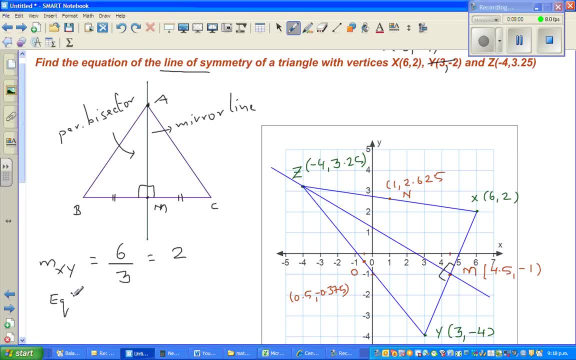 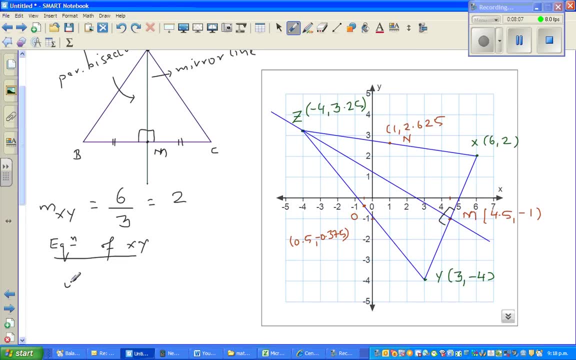 equation. so let me write equation of XY. okay, so you're using the gradient intercept formula. so Y is equal to 2, X plus C. now I can put either X or Y into this equation. so I know, on this line, when X is 6, Y is 2. so let me put this in this equation. so 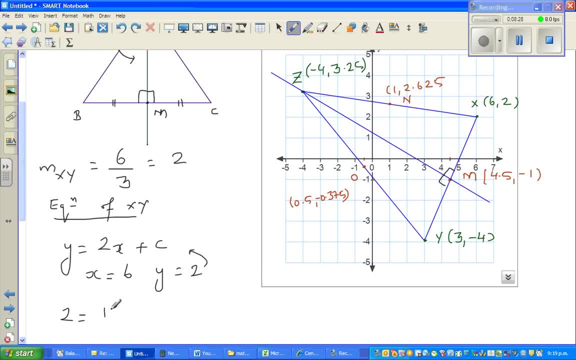 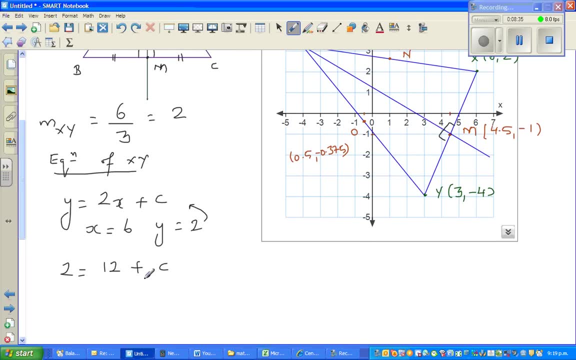 this becomes: 2 is equal to 12 plus C. how did they get it 12? that 2 times 6 is 12 and if you- I hope you understand- C would be negative 10 and it does make sense. the line intercept does make sense if. 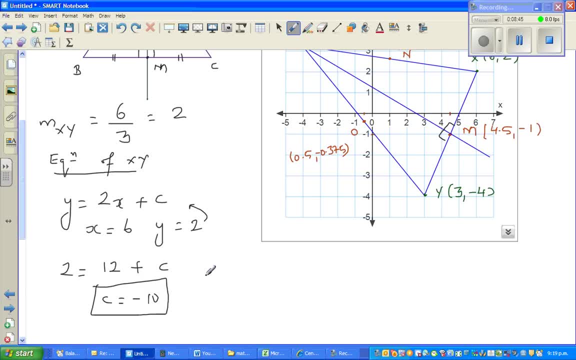 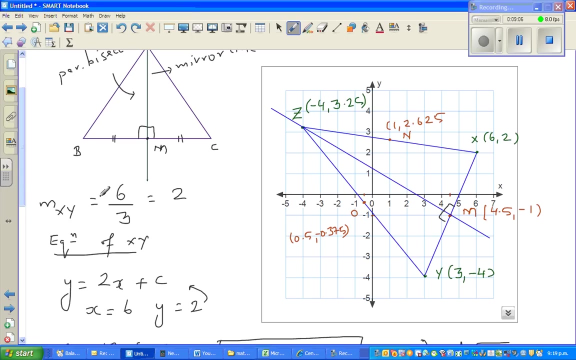 you extend this, this will cross the y-axis at somewhere, at negative 10. so the equation I can say: Y is equal to 2, X minus 10. so that's the equation of XY. this is the equation of XY, the line segment XY, so and so. equation of: 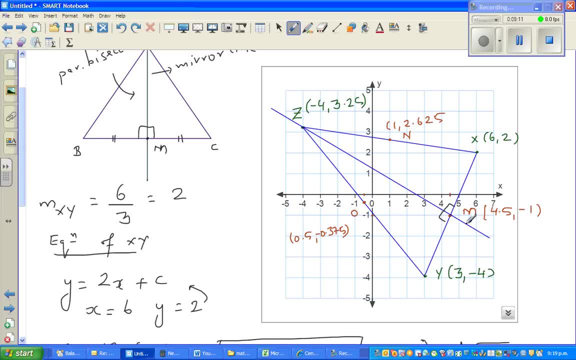 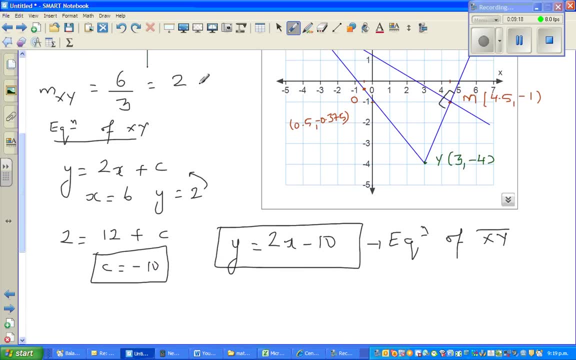 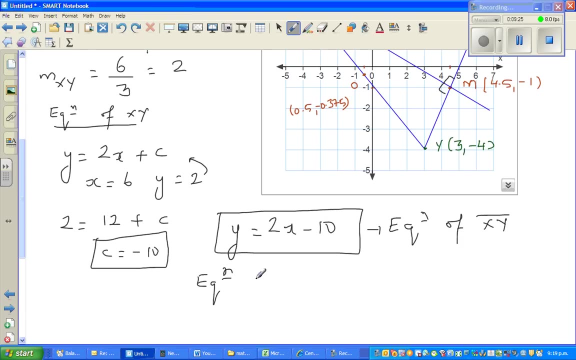 Now we want to find the equation. We didn't even need to find the equation of xy. if we had only found the gradient, that would have been good. So this is important, so you can ignore this, So we'll find. now we want to find the equation of zm. 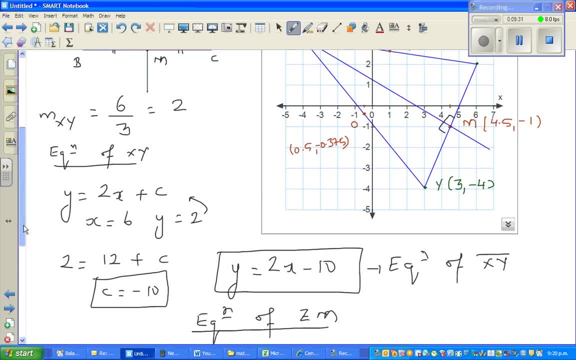 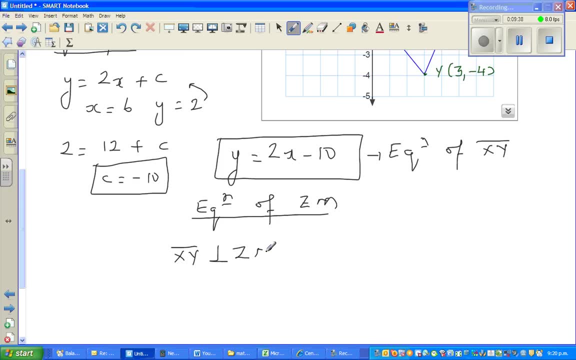 Equation of zm. Now I can say our xy is perpendicular to xm, which implies gradient of xy times. okay, I'll put the dot in algebra. it's good to put the dot because the x's will confuse. So xy, gradient of xy times the gradient of xm. 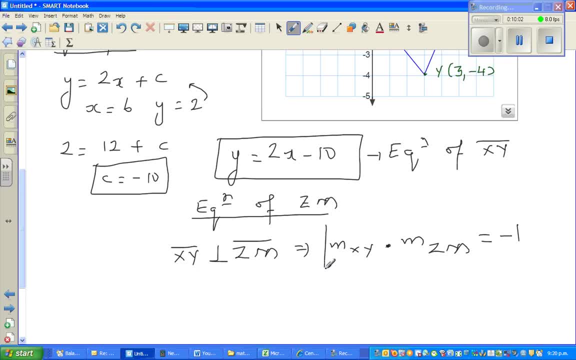 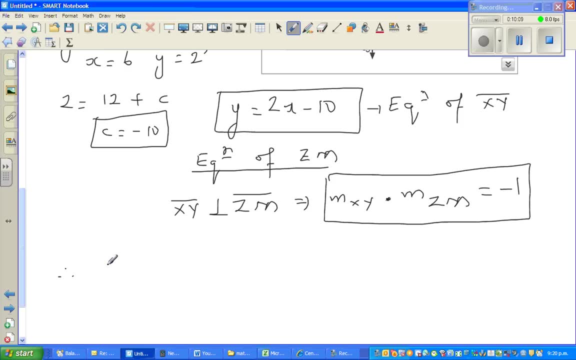 is the gradient of xm, So xy is negative 1.. So if two lines are perpendicular, the product of gradient is negative 1.. So I can say, therefore, m of xm would be negative 1 half. Why? Because 2 times negative 1 half gives you negative 1.. 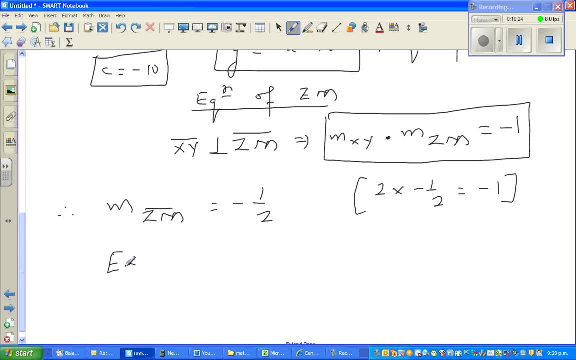 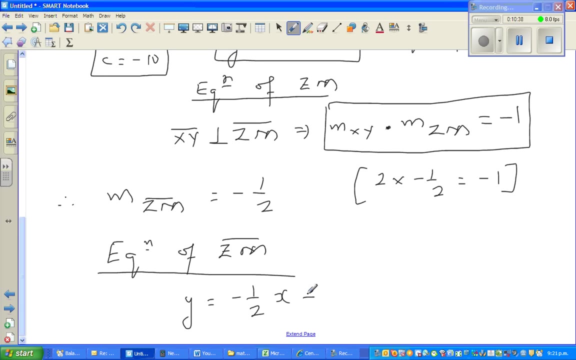 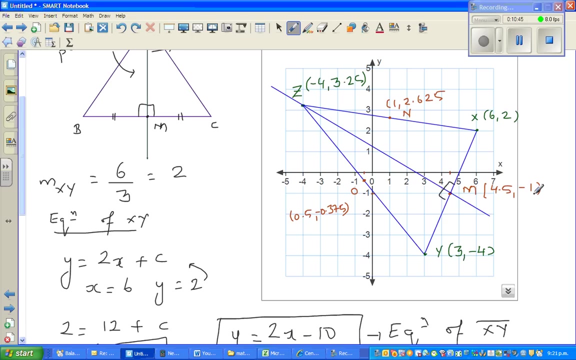 Okay, so equation of zm. I'm trying to finish it off soon. So y is equal to negative 1 half x plus c. Okay now, which point can I put here? I can put this point of 4.5, negative 1.. 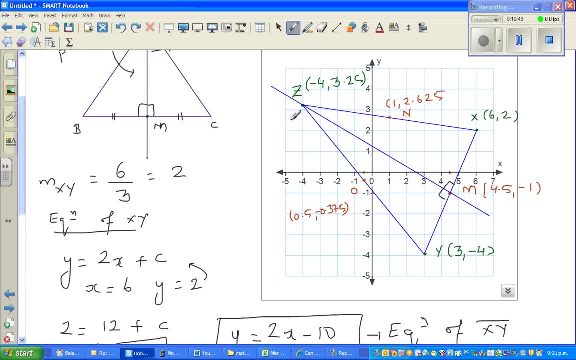 Okay. so I know I'm not sure about this, but I'm making a guess. But I surely know that this line is passing through the midpoint of xy. So when x is 4.5, y is negative 1.. So let me change color. 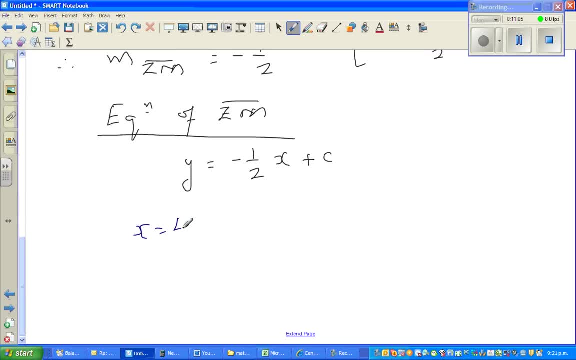 I can say when x is 4.5, y is negative 1. So negative 1 is minus half times 4.5 plus c. So negative 1 is half of 4.5, is negative 2.25 plus c. 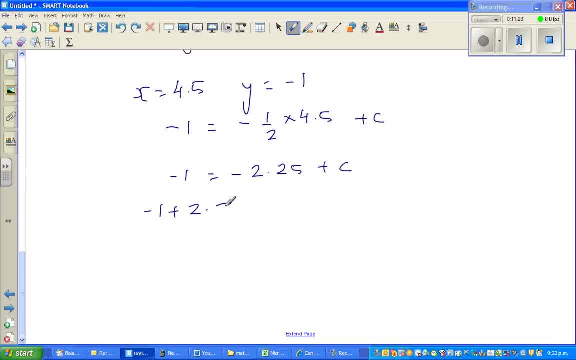 So minus 1 plus 2.25.. So y is equal to c, which implies c is 1.25.. So let me write the equation of zm. Am I right? Equation of zm is y is equal to equation of zm. I should not write 2 equal to. 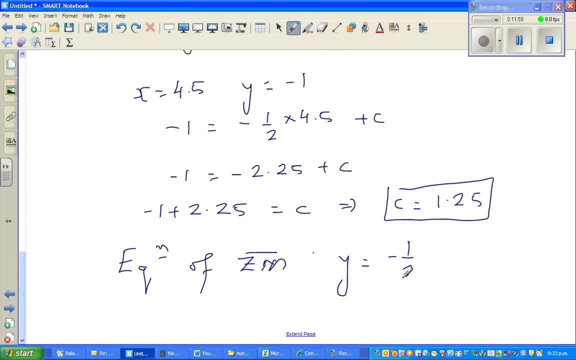 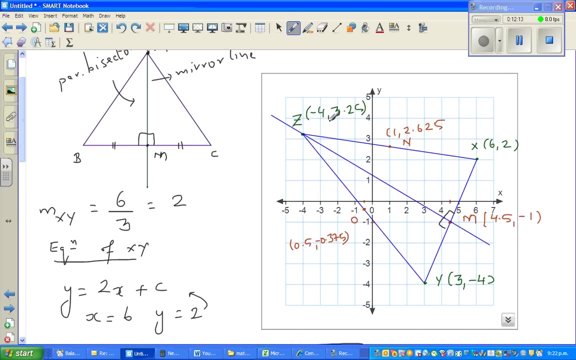 so y is equal to negative 1, half x plus 1.25,. that's what I'm saying. Now, to show that this is a line of symmetry, I have to show that this passes through this point. Okay, so if you can save, so when x is minus 4,. 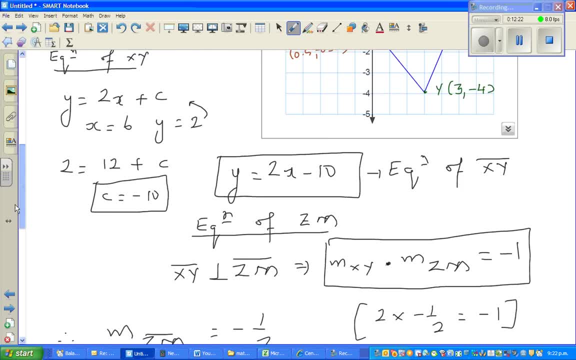 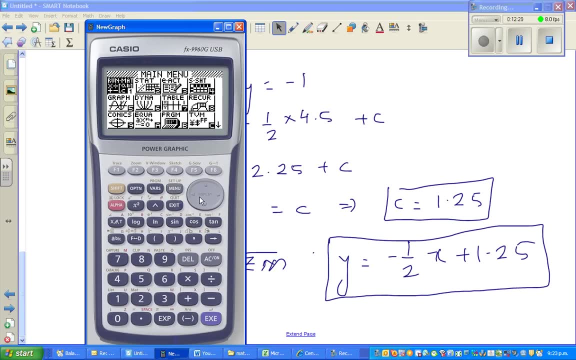 minus 4, y should be 3.25.. So I'll use the calculator. You can do without the calculator, but I want to finish it off soon, So let me graph the equation. So let us go to graph and type in this equation of y. 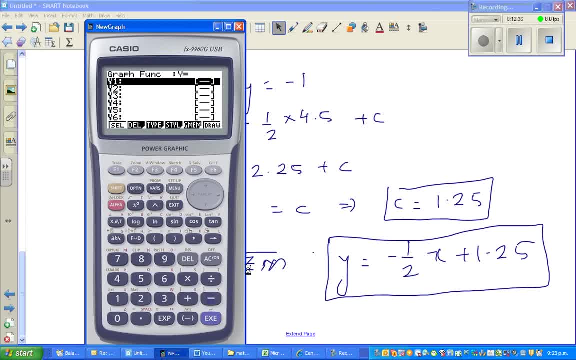 So minus 0.5, so I can write minus 0.5x plus 1.25.. Okay, and then draw it And then you go gsolve when you want to find y calc when x is what was the value of x? 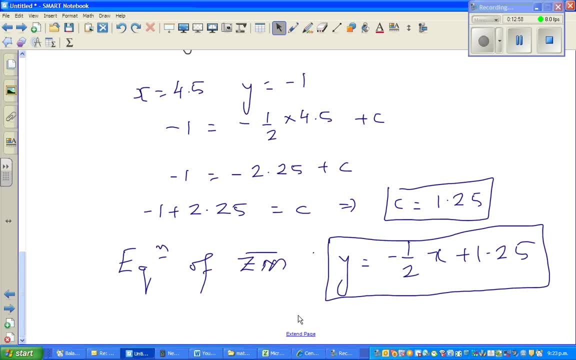 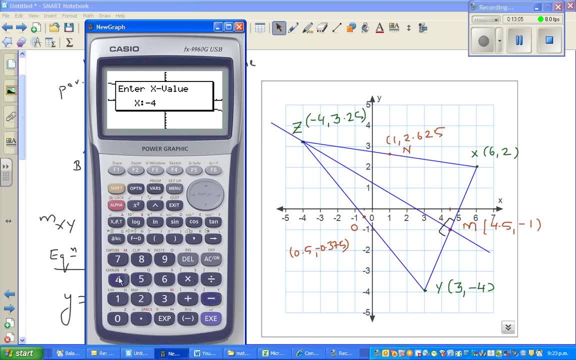 So y is equal to 0.5x plus 1.25.. Okay, So I forgot that. so it's always good to show When x is negative 4, when x is negative 4, what's y? So there we go. 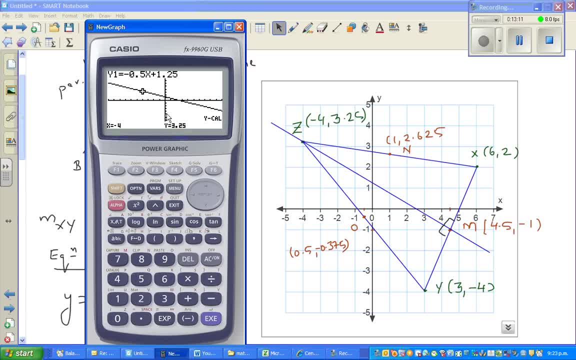 When x is negative 4,, y is 3.25, because- and that's what the graph tells me- that this line, or this point lies on this line. Okay, So we can say now: now, when x is negative 4,. 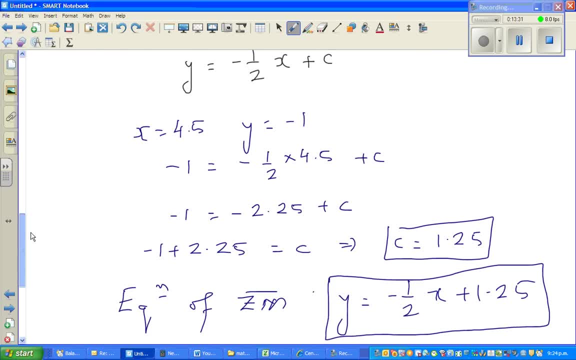 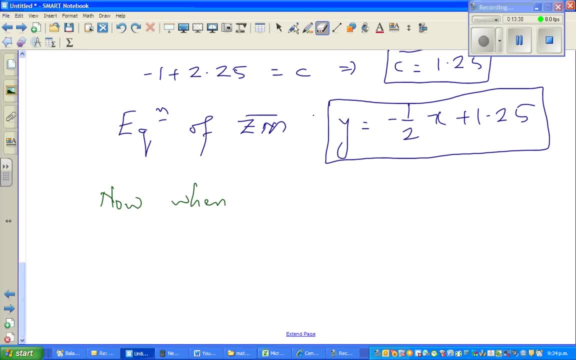 when x is equal to. when x is negative 4, when x- let me write that better- when x is equal to negative 4, y is equal to. I keep forgetting the values. When x is negative 4, y is minus 3.25,, which implies that z lies. 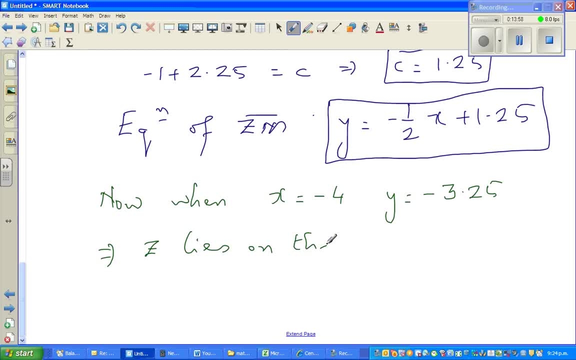 on y. Okay. So how many times can we say that? oh, we have x. So when x is negative, 4, y is very similar to negative 4.. Okay, And this is 0.5x minus 2..